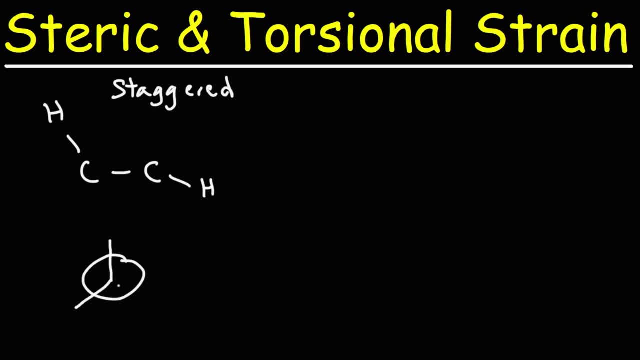 If you draw the noon projection, it would look like this: So if we were to draw ethane, we would draw a staggered conformation. Let's color code these hydrogen atoms. So let's make this a red hydrogen atom and we'll make this a blue one. 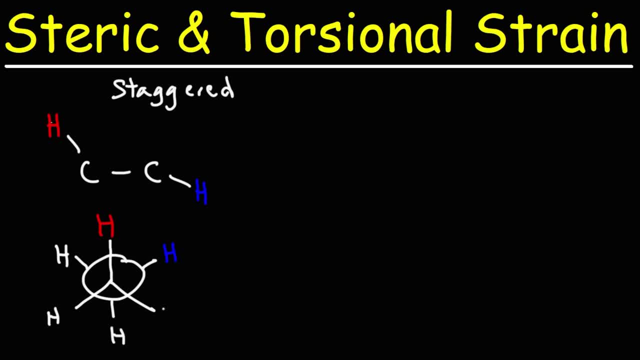 So those two hydrogen atoms are in a staggered conformation. They're not eclipsed at this point. Now what we can do is we can rotate the backside so that we can get an eclipsed conformation. The noon projection will look something like this: 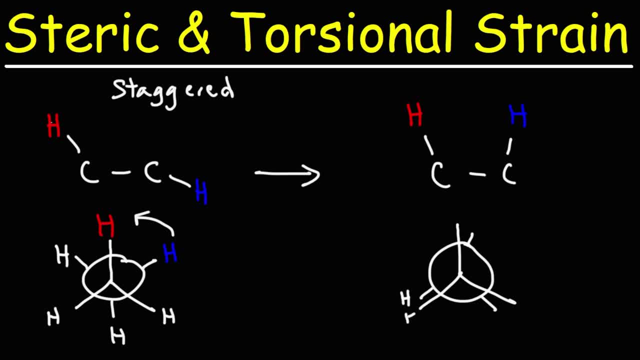 So the blue hydrogen is behind the red hydrogen, if you see it from this side. So that's the eclipsed conformation. The torsional strain exists due to the electron repulsion That's in the CH bonds, The electrons there they're going to repel each other. 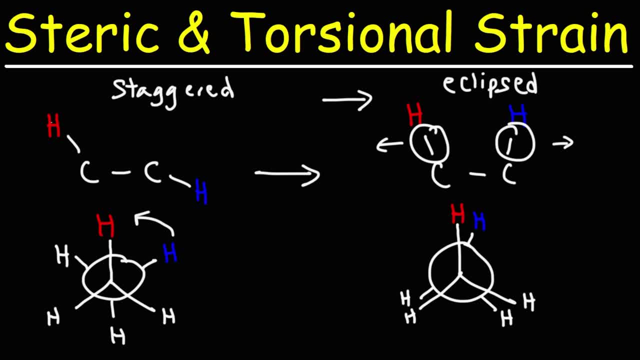 And so you're going to have that torsional strain. The eclipsed conformation is less stable, which means it's at a higher potential energy, And the staggered conformation: it's more stable, which means it's at a lower potential energy. 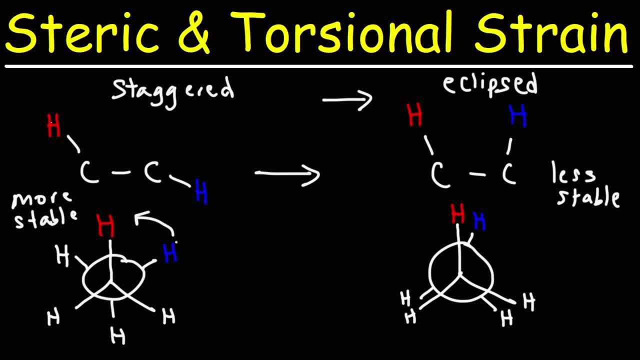 So when you try to rotate the bond, in this case this particular carbon-carbon bond, to go from the staggered to the eclipsed conformation, ethane doesn't want to be an eclipsed conformation. This is a relatively unstable conformation. 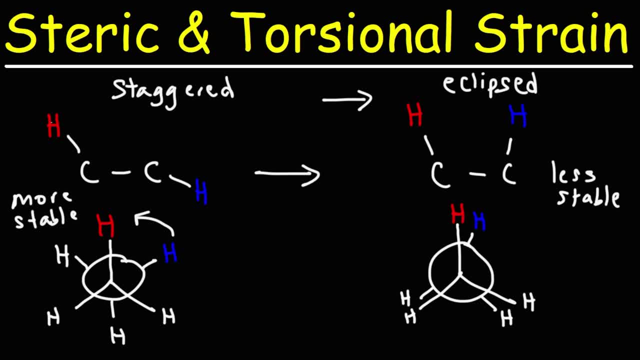 So as you try to rotate it, you're going to experience resistance to rotation, And that resistance is the torsional strain that arises from the repulsion of the electrons in the CH bonds, in ethane in this example. So think of torsional strain as 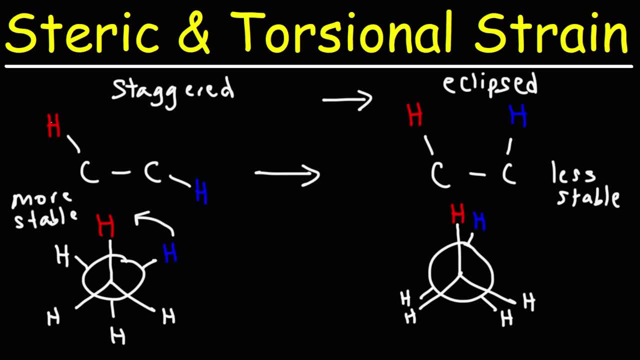 an eclipsing strain. Anytime you have atoms that are eclipsed from each other, you're going to have that torsional strain. Now, the torsional strain, it's found in the bonds of atoms that are three bonds apart. So here's one bond, two bond, three bonds. So it's going to be found in these bonds. 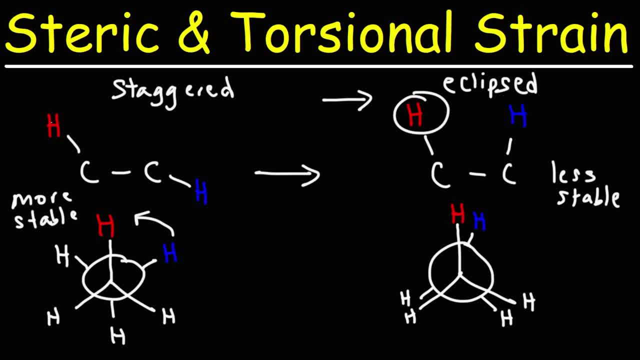 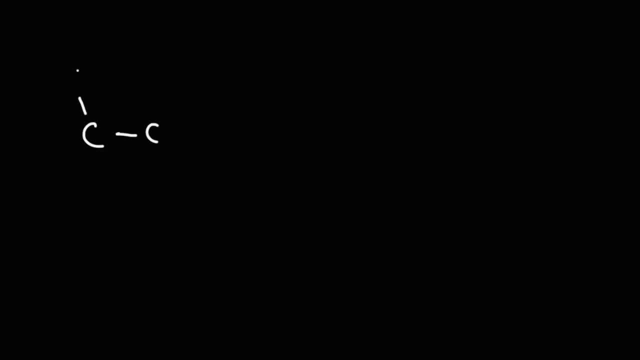 Steric strain can be found between atoms that are more than three bonds apart. So here's an example of when you'll get steric strain, particularly when you have two bulky groups next to each other. In this case, we have two bulky methyl groups. 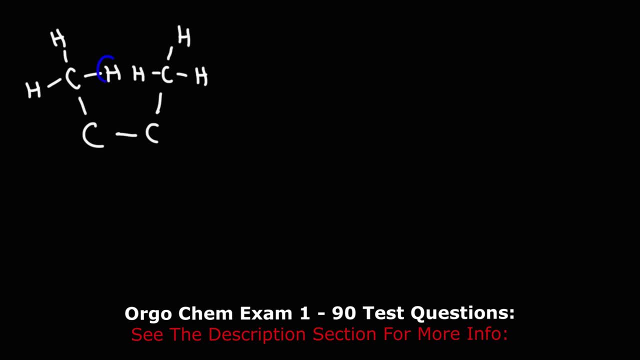 Notice that the electron clouds of the hydrogen atoms. they're very close to each other And, as we know, when you place two electrons next to each other, light charges, they repel, And so they're going to feel an electrostatic force. 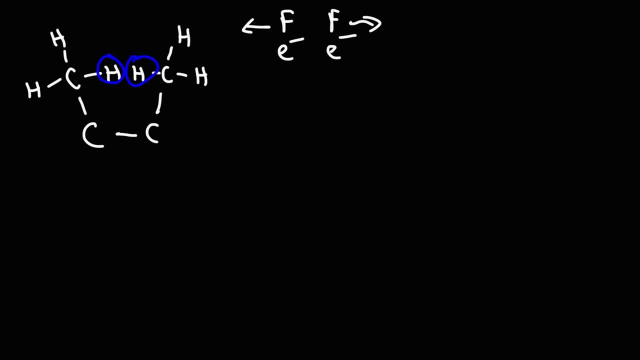 Let me say that again- an electrostatic force of repulsion. So that's when you'll have steric strain. Typically, whenever you have bulky groups next to each other, it's going to be steric strain. And if you count the bonds between those two atoms, they're more than three bonds apart. 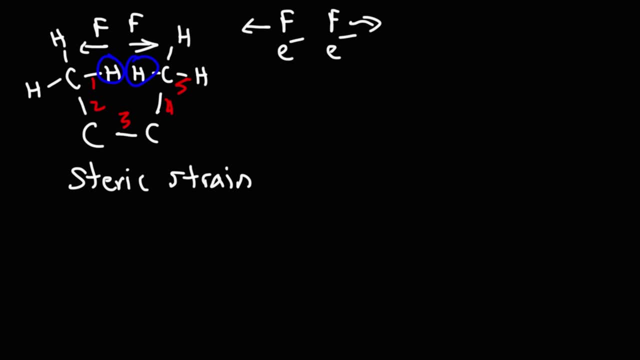 So that's the difference between torsional strain and steric strain. Steric strain arises from when atoms get close to each other and their electron clouds repel each other. Torsional strain has to do with the electrons: The electrons and the bonds that repel each other whenever you have an eclipse conformation. 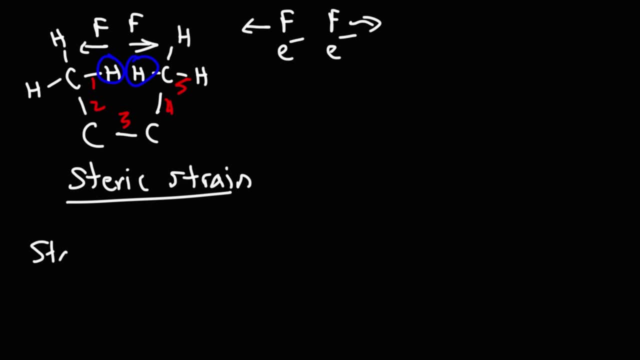 Steric strain. it can be present in a staggered conformation or an eclipse conformation. Torsional strain is only found in eclipse conformation. So if you have a staggered conformation, there's not going to be any torsional strain. 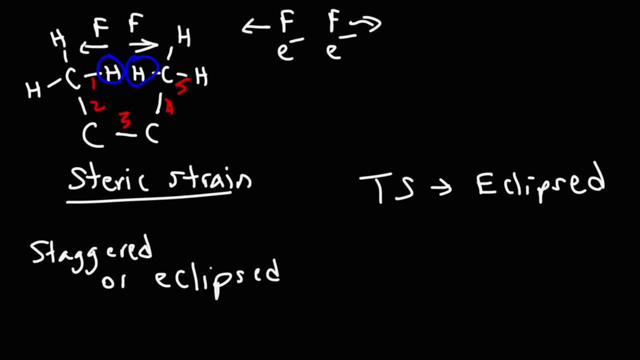 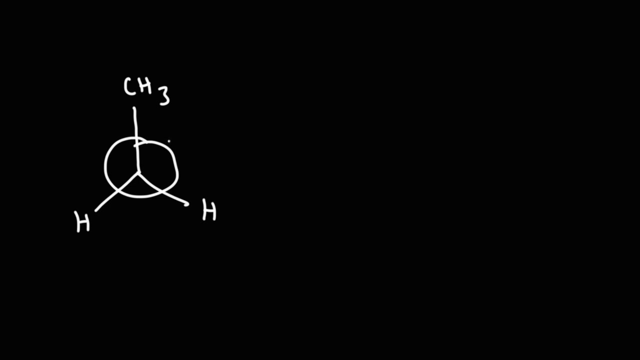 And that's how you can easily identify when there's torsional strain. Look for the eclipses. So this is the eclipses conformation. Let's go over some examples Here. we have a Newman projection, And this is going to be of two methylbutane. 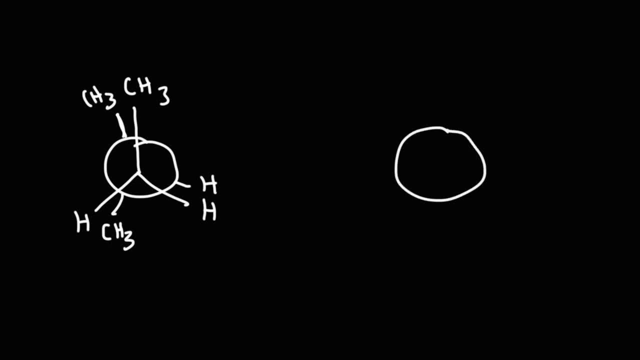 And let's compare it with this one. So which one is the eclipse conformation and which one is the stagger conformation? On the left we have the eclipse conformation. On the right, we have the staggered conformation. Now, looking at the interactions in these conformations, would you say there's torsional strain steric. 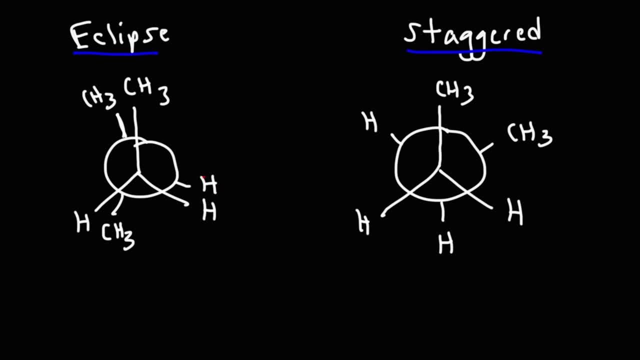 strain or both. So here we have two hydrogen atoms that are eclipsed to each other. We're going to have torsional strain there. Anytime you have an eclipsing interaction, there's going to be torsional strain. Here we have a hydrogen and a methyl eclipsing each other. you're going to have torsional. 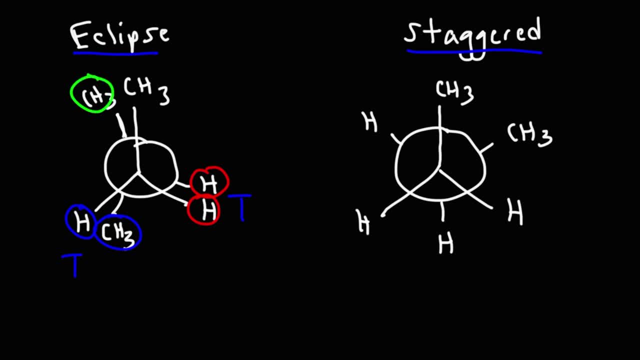 strain. Here we have two bulky groups, two methyl groups that are eclipsing each other, So that's going to have torsional strain as well. In the stagger conformation there is no torsional strain. The hydrogens- they're too far apart. 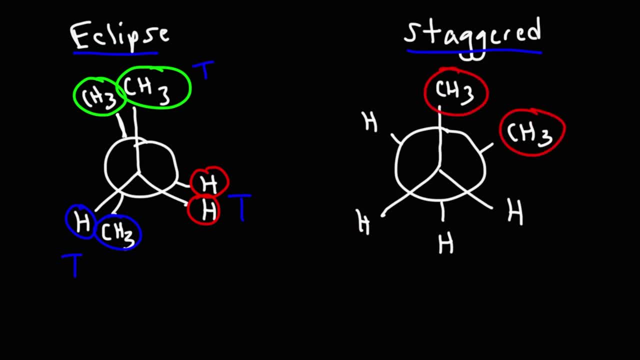 Even these two methyl groups. There's no torsional strain between them. However, there is a special interaction, which is known as the Gauch interaction, And whenever you have two bulky groups that are 60 degrees apart, you're going to have 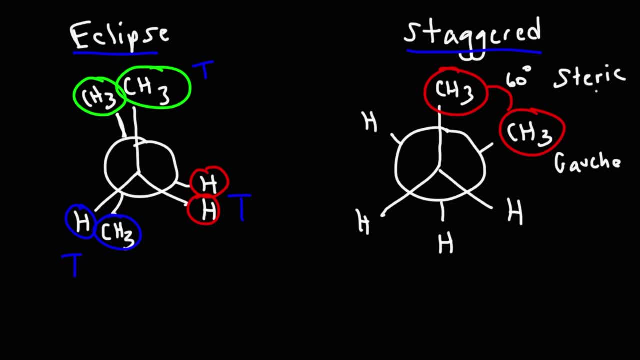 steric strain. So steric strain does exist in the stagger conformation if the two bulky groups are within 60 degrees apart. Now here the bulky groups are next to each other in this eclipsed conformation, So in addition to torsional strain you also have steric strain here. 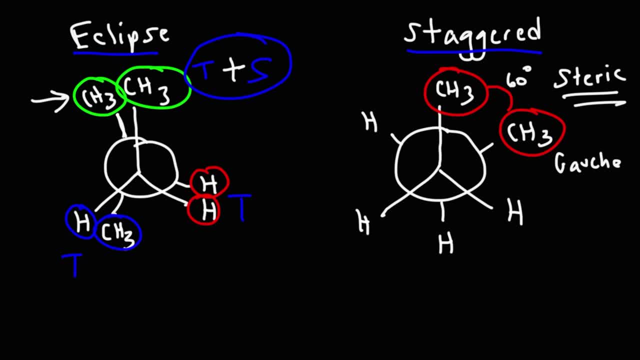 So, to keep things simple, if you're taking an organic chemistry exam, remember anytime you have an eclipsed conformation, you're going to have torsional strain, And anytime you have two bulky groups next to each other, you're going to have steric. 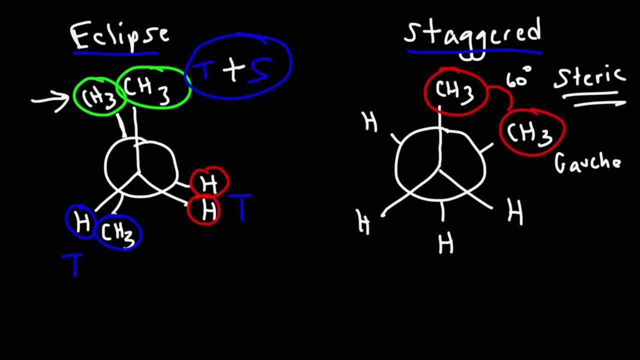 strain. Okay, Now the energy values. the relative potential energy for two hydrogen atoms eclipsed in each other is four kilojoules per mole. For hydrogen and methyl it's six. For two methyl groups it's 11.. 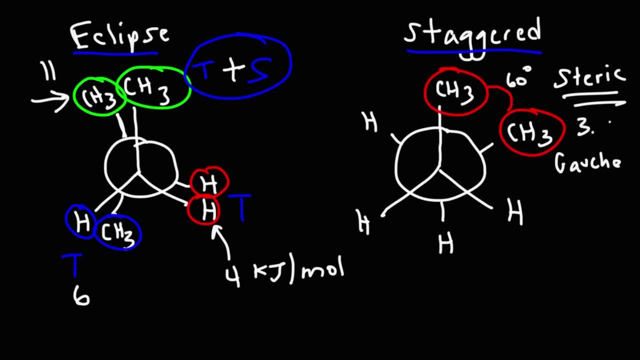 Now for the steric interaction between two methyl groups. the energy for that is 3.8.. Okay, Now here's a question for you. Why is it that the hydrogen-hydrogen eclipse interaction, why does it have more energy than the two CH3s in the Gauch interaction? 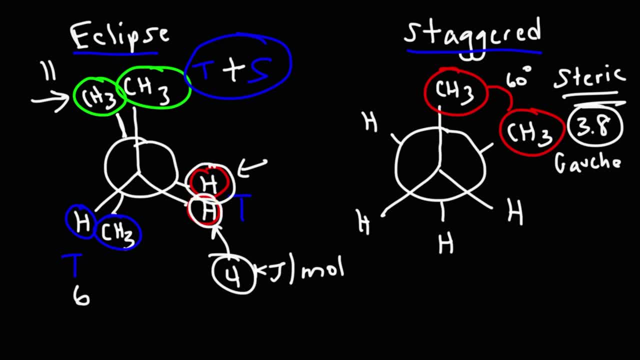 Especially given the fact that these atoms are smaller than the methyl group. they're less bulkier. why does it have a higher potential energy? The reason: Even though, Even though these atoms are smaller, they're much closer. These atoms are bigger, but the bonds in the atoms, they're farther apart. 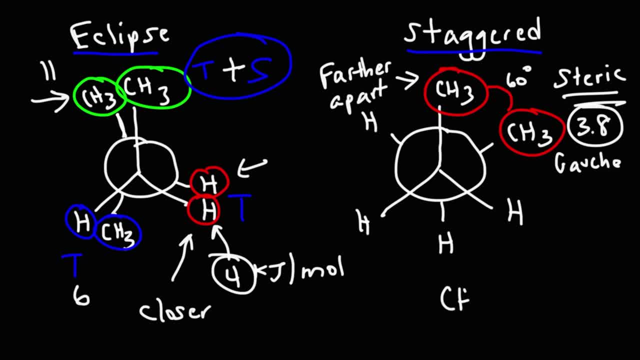 And so that's why the two methyl groups in a staggered interaction have less potential energy than the two hydrogen atoms that are in the eclipse interaction is because in the eclipse interaction it's much closer compared to the steric interaction. Okay, Okay. 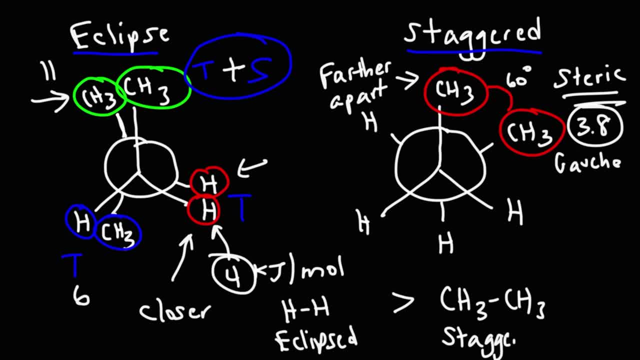 All right, Yeah, So that's the first more complex thing to do In theики of intergalactic attraction. we'll be going through a lot of these. Okay, Okay, All right. So this is. it's the third-most complex thing we're gonna focus.